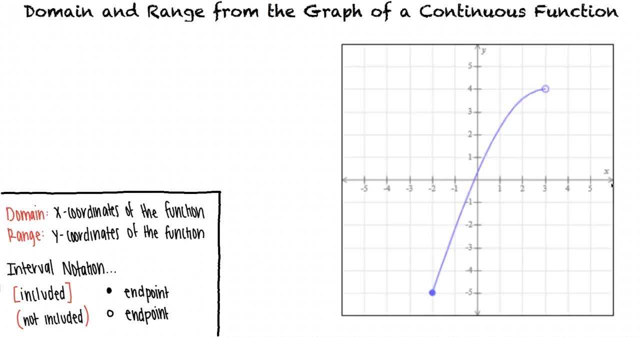 we want to examine the function from left to right. We see that the leftmost x coordinate is negative 2, and that the endpoint is a filled-in circle. This means we'll use a bracket to indicate the smallest value of x, to indicate the smallest value in our domain. 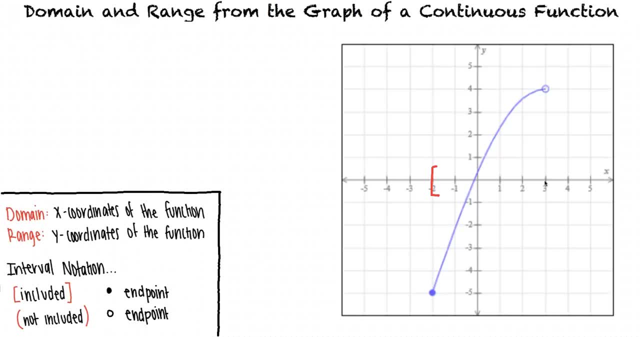 The rightmost x coordinate is 3,. however, this endpoint is an open circle. This means that the x coordinate 3 is not actually included in the domain, but the x coordinates get infinitely close to 3 without ever being 3.. This tells us: we'll use a parenthesis in our notation. 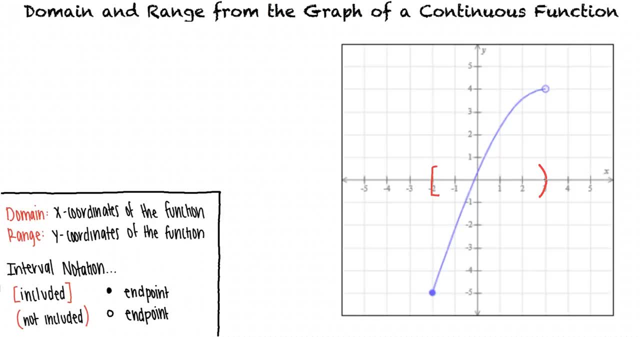 Between the x coordinates, negative 2 and 3, there are no other holes or breaks in the function, which tells us that the domain includes all values greater than or equal to negative 2 and less than 3.. We write this in interval notation as: 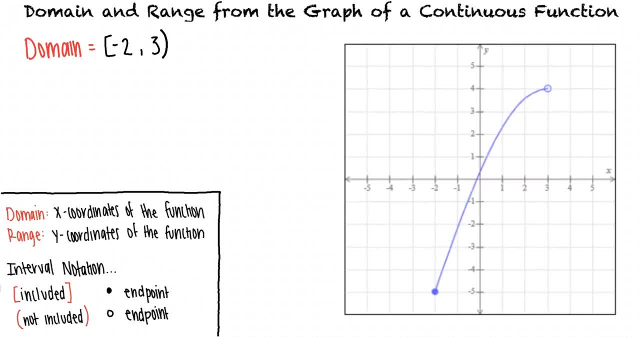 Now let's determine the range, Since range deals with y values, which corresponds to the y-axis. we now want to examine the graph from bottom to top. We see that the bottommost y coordinate is negative 5, and the endpoint is a filled-in circle. 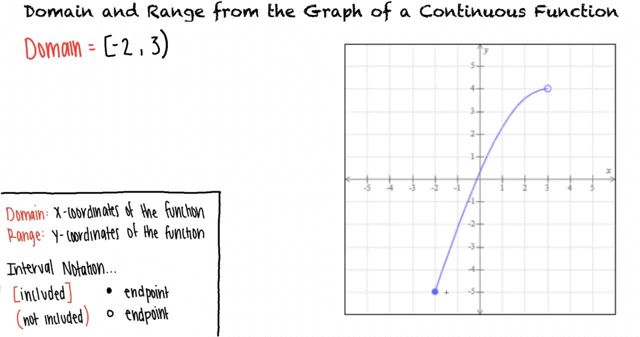 This means we'll use a bracket to indicate the smallest value. in our range, The topmost y coordinate is 4,. however, this endpoint is an open circle. This means that the y coordinate 4 is not actually included in the range, but the y coordinates get infinitely close to 4 without ever being 4.. 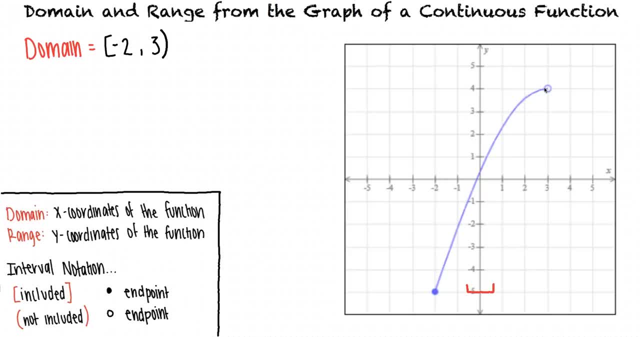 This tells us. we'll use a parenthesis in our notation. Between the y coordinates negative 5 and 4, there are no holes or breaks in the function, which means that the range includes all values greater than or equal to negative 5 and less than 4.. 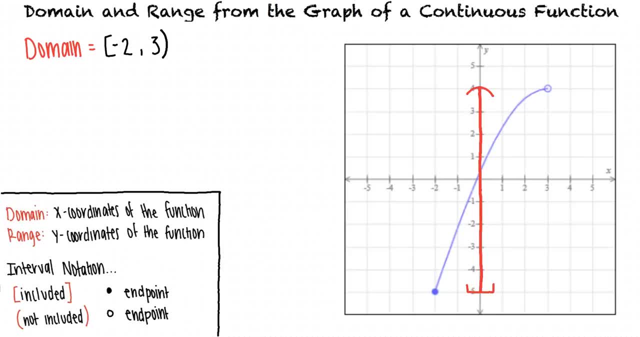 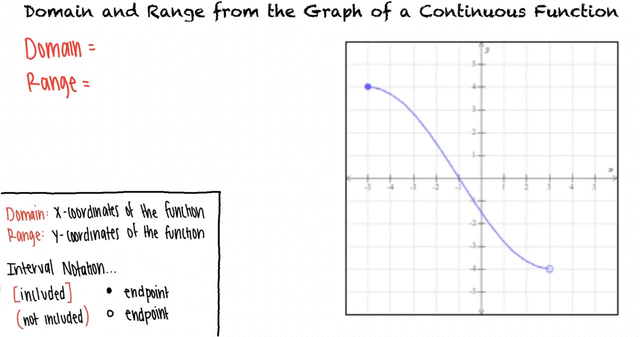 We write this in interval notation. as Let's take a look at another example. How do you think we should go about finding the domain and range of this function? If we start with the domain, we need to look at the x values included in the function.